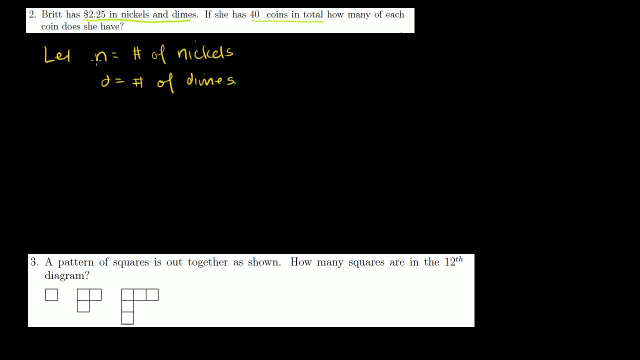 and dimes. So how much money does she have? Well, if you take the number of nickels, each nickel is worth $0.05.. So the number of nickels times 0.5.. 0.05, that's how much money her nickels represent plus. 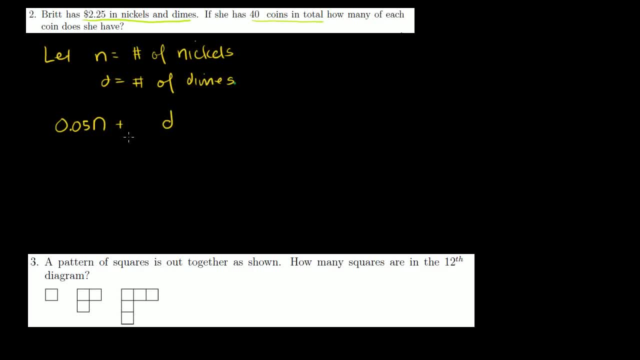 the amount of money her dimes represent. So she's got d dimes. They're each worth 0.1 of a dollar, or 0.10, if we want to put the 0 in front of the decimal. So this is the total amount of money she has right. 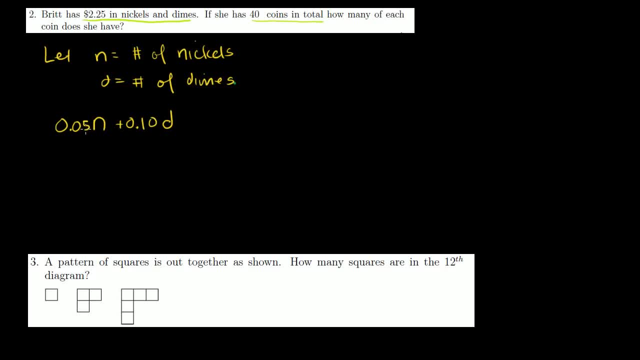 If she has 5 nickels, you'd do 5 times 5 cents, It'd be 25 cents. If she had 4 dimes, that'd be 40 cents And you would add it all together. Now the problem tells us that the 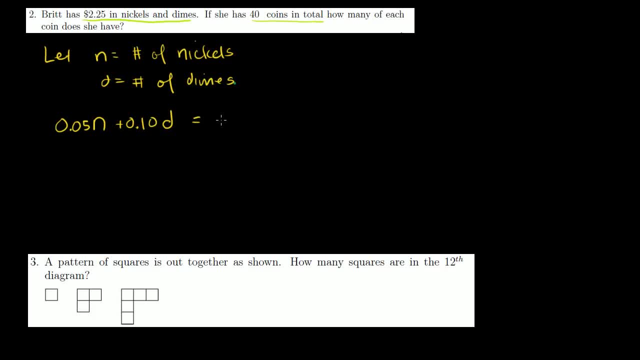 total amount of money she has is $2.25.. So this first statement right there can be translated into this equation right here. She has a certain number of nickels and a certain number of dimes. You multiply 5 cents times the nickels plus 10 cents times. 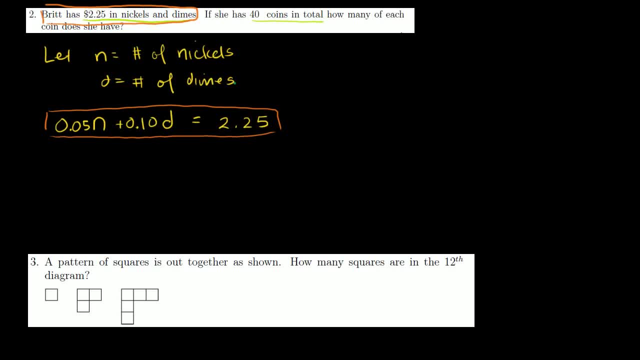 the number of dimes, You can end up with 225.. Now this second statement. she has 40 coins in total And I'm assuming that she only has nickels and dimes, that there aren't any other coins. So 40 coins in total. that means that the number of 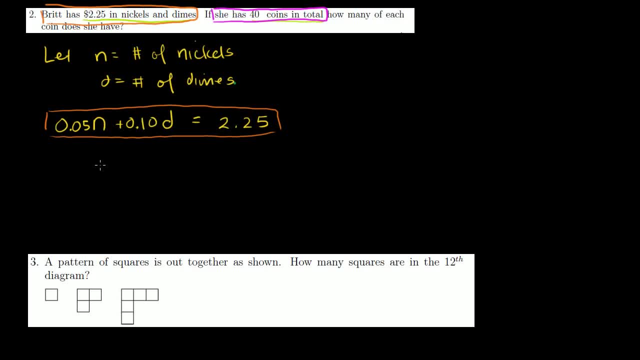 nickels plus the number of dimes has to be equal to 40. So the nickels plus the dimes has got to be equal to 40. That's what that information tells us. Now we have two equations with two unknowns. 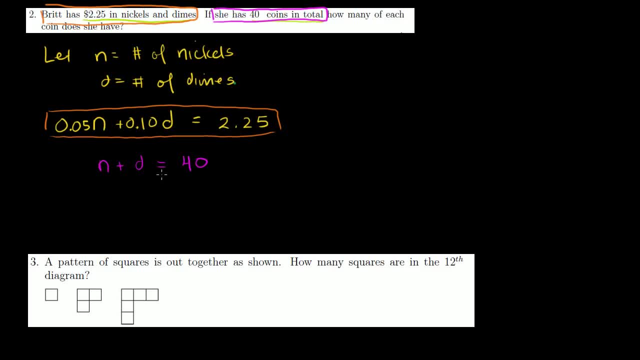 And there's two ways we can do this. We can do this as a system and we can subtract one equation from the other, Or we could do substitution. Let's do substitution. That's often a more intuitive way to do it. So what I'm going to do is I could solve for either one. 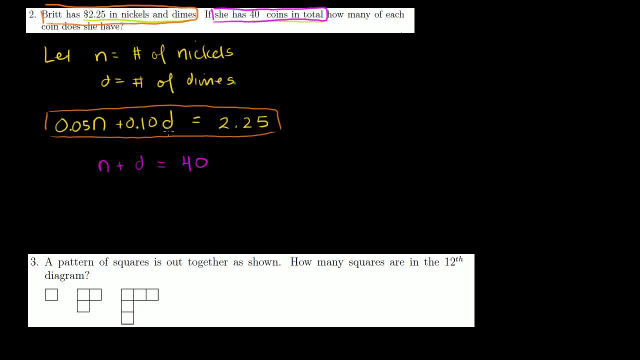 But I'll solve for d and then I'll substitute whatever I get for the d in this equation right here. So if we subtract n from both sides of this equation, so let me do that- Negative n plus this minus n. Obviously these cancel out and you're just left with d. 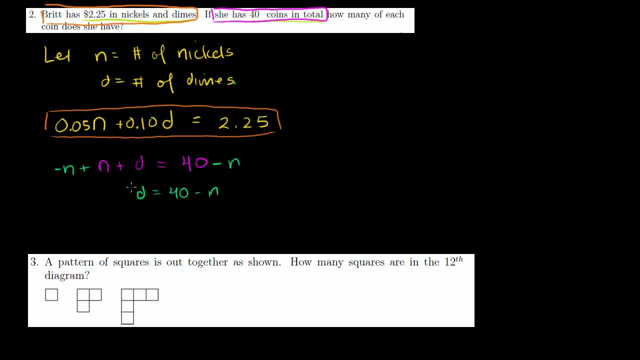 is equal to 40 minus n. Now we can take this. We just established, using the second equation, using this second statement, that d is equal to 40 minus the number of nickels And we can use that to substitute back in for d. 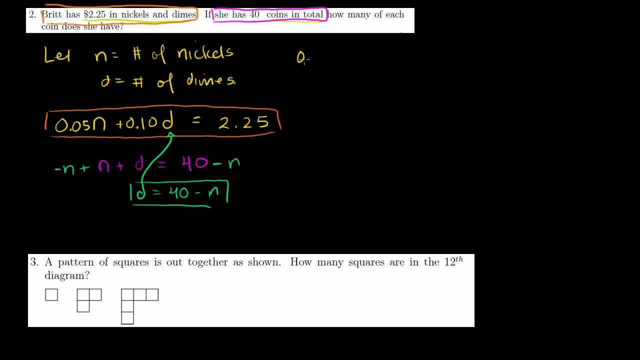 So this first equation will now become 0.05 times our number of nickels, plus 0.1 times our number of dimes. We already know the number of dimes is equal to 40 minus n. That's what that second statement is. 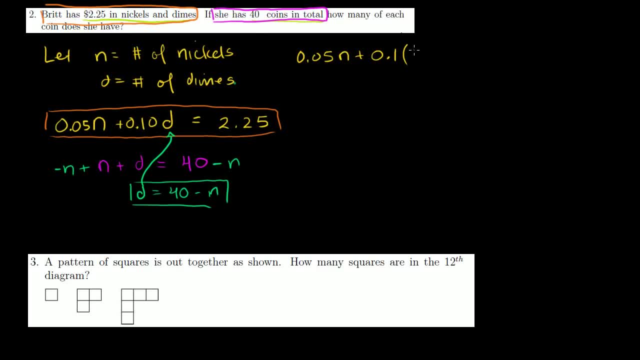 That's what that second statement told us. So instead of d, I'm going to substitute it with 40 minus n. That's the number of dimes we have, It's 40 minus the number of nickels, And that is equal to $2.25.. 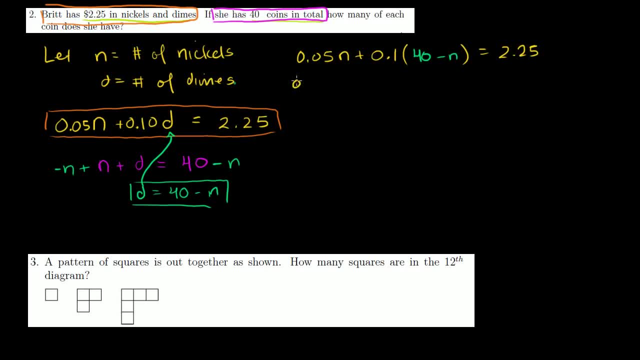 And now we can just try to solve for n. So we get 0.05n plus 0.1 times 40.. That is 4.. Let me show you that I'm distributing it, So 0.1 times 40.. 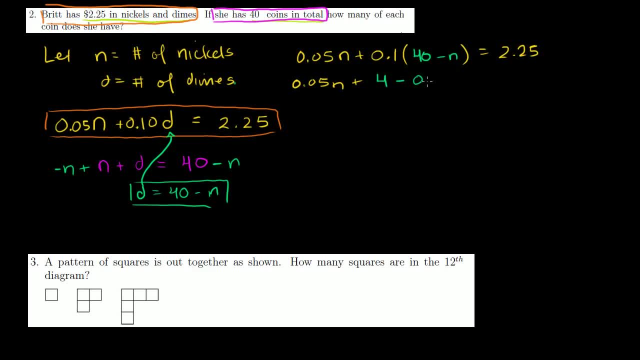 That is 4. Minus 0.05n. That is 4. Minus 0.05n, Minus 0.05n Minus 0.1n. I just distribute this times each of these terms. 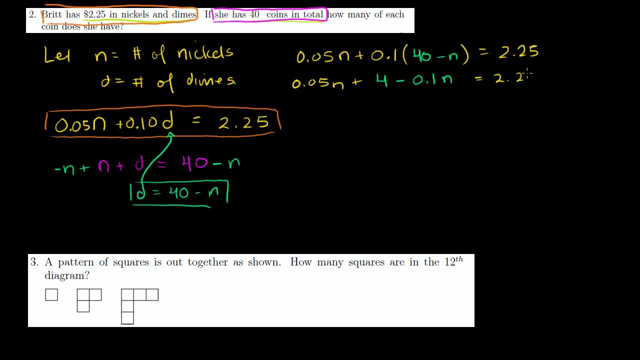 Is equal to $2.25.. And then, what can we do? Well, we can take 0.05 minus 0.1, or 0.10, depending on how you want to do it. If you take those two terms, you're actually. 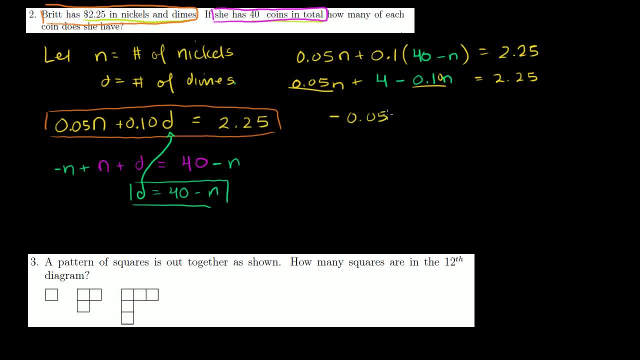 going to get a negative 0.05n. 0.05 minus 0.10.. This is twice as big as that, So it's going to get a negative number Plus 4.. So I still have that 4.. 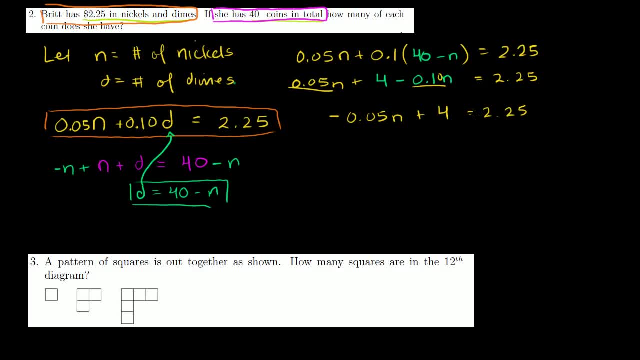 Is equal to $2.25.. Now I can subtract 4 from both sides of this equation. I get negative. 0.05n is equal to: if you subtract 4 from the left, that 4 is going to go away. 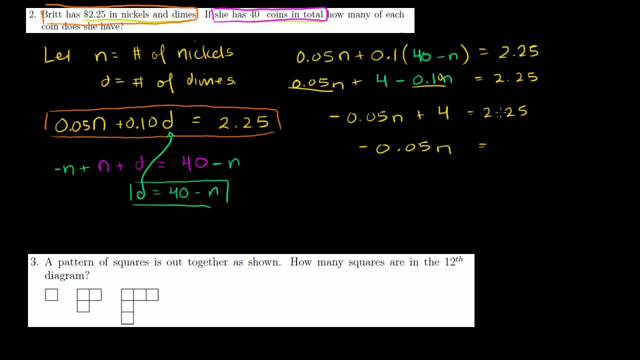 You subtract 4 over here: 2.25 minus 0.05n Minus 4. That's negative 1.75.. Now we can multiply both sides of this equation by negative 1, just to make it a little bit cleaner. 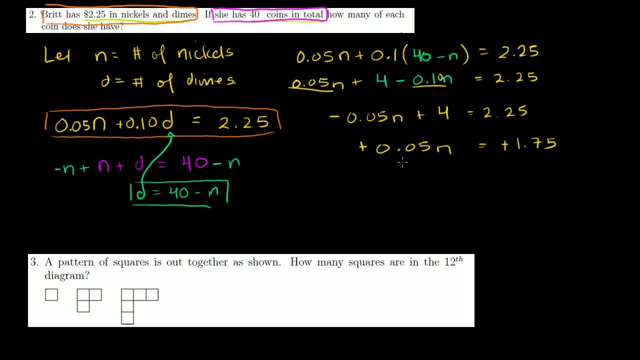 So that becomes a plus and a plus, And then divide both sides by 0.05.. I could have just divided both sides by negative 0.05 to begin with, But I like getting everything positive. So if you divide it by 0.05, you get n is equal to 0.05n. 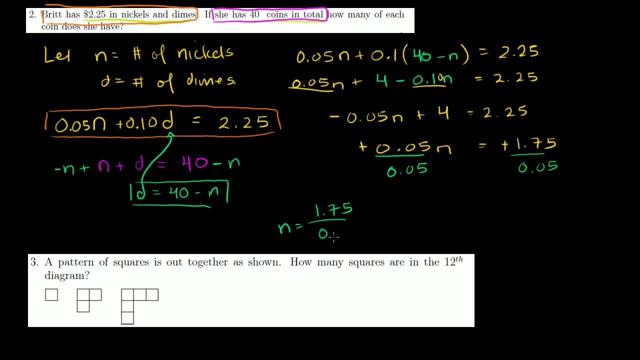 Let's do it in a different color. So let's do this division. Let me do it in a different color: 0.05 divided into $1.75.. Let's multiply both the divisor and the dividend by 100.. So we're going to go over two decimal spaces. 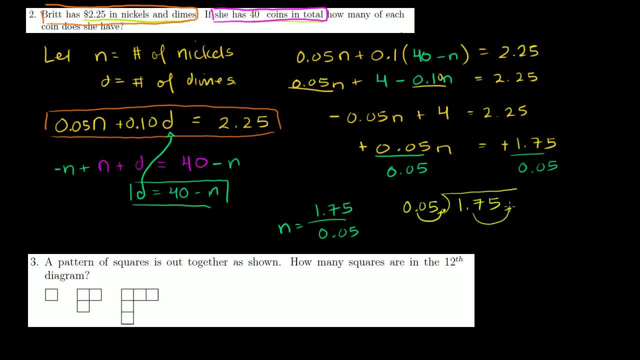 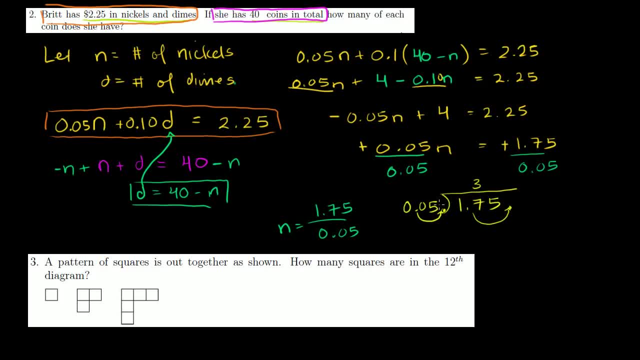 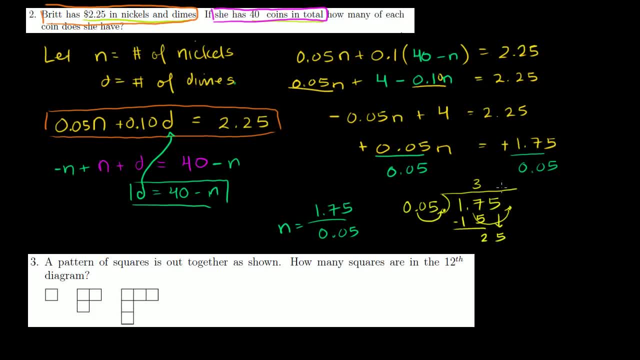 Bring down the 5. 25. 5 goes into 25. five times 5 times 5 is 25.. You have no remainder. So this is equal to 35. So n is equal to 35.. Now we could solve for d. 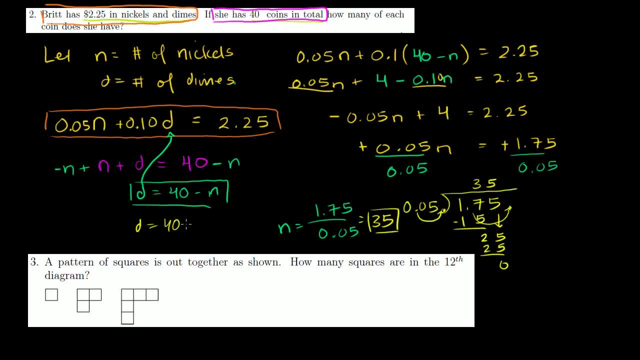 d is equal to 40 minus n, So d is equal to 40.. minus 35,, which is equal to 5.. So we have 5 dimes and 35 nickels, And just to verify that that actually does make sense. 35 nickels are going to be worth how much? Well, 35 times 5 cents is going to get us to 175 cents, or $1.75.. So this times 35,, that is going to be $1.75. 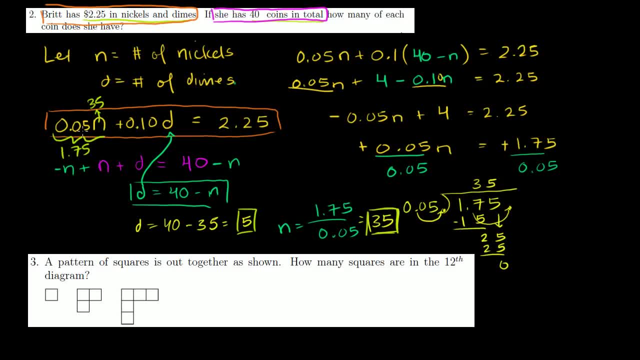 $1.75 in nickels, 35 times 5, or times 0.05,, depending on how you view it, And then this is going to be 5.. So this right here is going to be 50 cents in dimes. 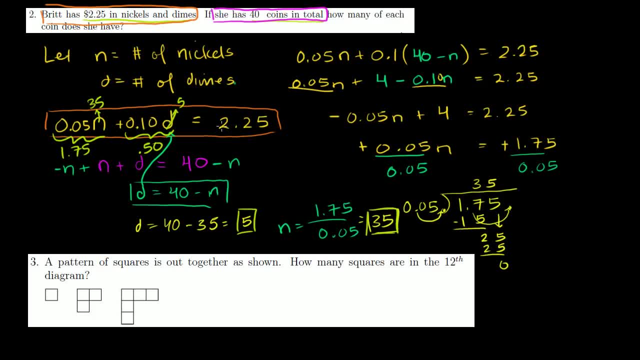 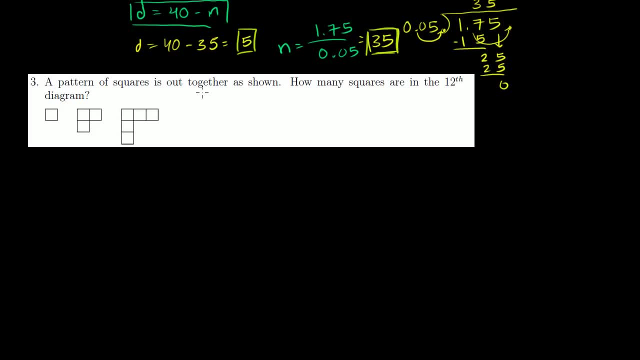 $1.75 plus 50 cents, that's 225.. Let's do one more. A pattern of squares is out together as shown. I guess they're hanging out How many squares are in the 12th diagram. So let's see what's happening. 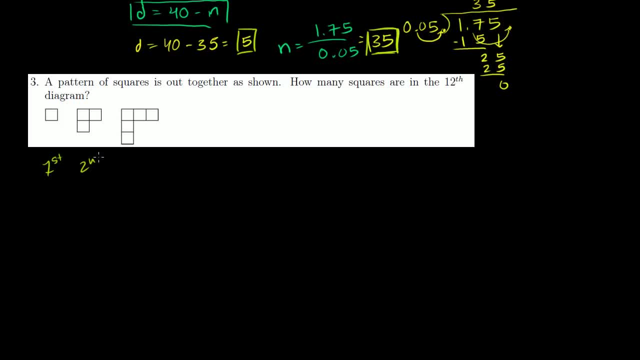 So this is the first, That is the second, That is the third. Let's see here: Each side, this is a 1 by 1 square, And then here it's 2 by 2.. But then they take out this block right over there. 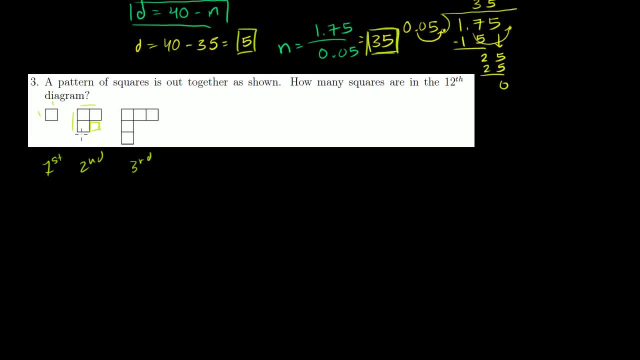 So let's see. So one way you could think about it is: this is 2 by 2.. Now, this is a 3 by 3. But they took out the 2 by 2. And so the next one is going to be. 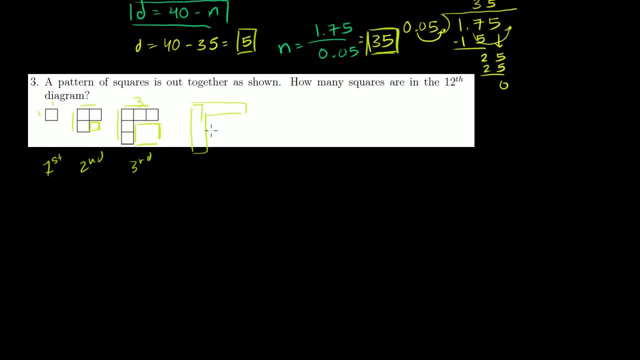 a 4 by 4, where they took out the 3 by 3.. So I guess one way that we can describe the number of squares- actually the easiest way I didn't have to think about that- is: look, I have 3 here. 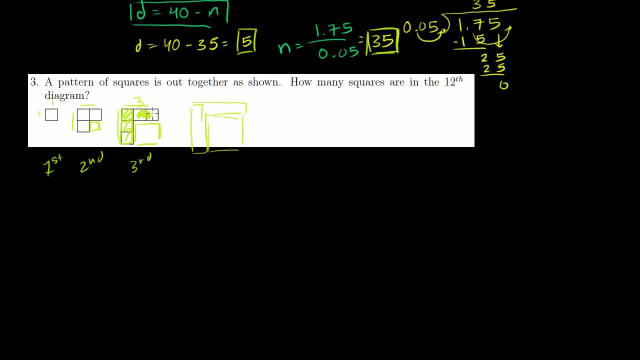 And then I have 3 minus 1 over here. Let me do that in a different color right. 3 minus 1 over here. Here I have 2.. And here I have 2 minus 1.. And then here I have 1.. 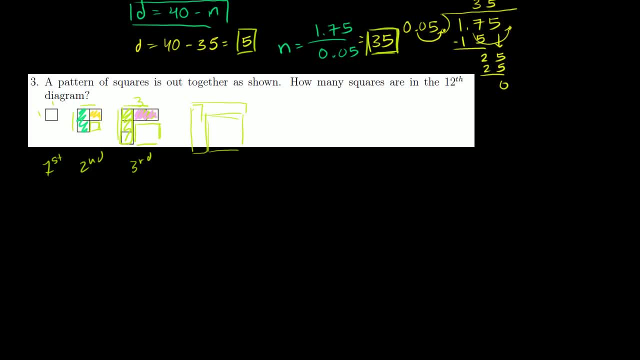 And then here I have 1 minus 1.. I have nothing. So in general the number of squares for any n is going to be n plus. then we have n minus 1, plus n minus 1, which is the same thing as 2n minus 1.. 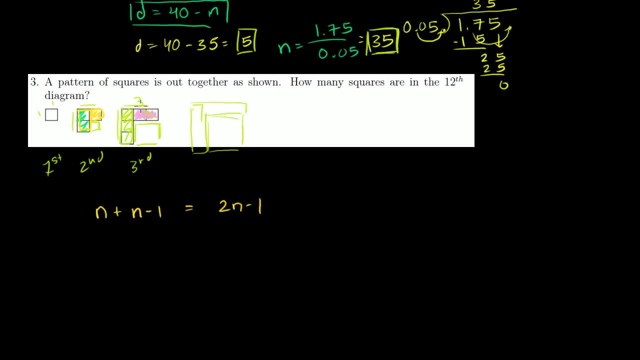 And it works right: 2n minus 1.. 2 times 3 minus 1. Minus 1 is 5.. 1,, 2,, 3,, 4,, 5.. So it works for these 3.. 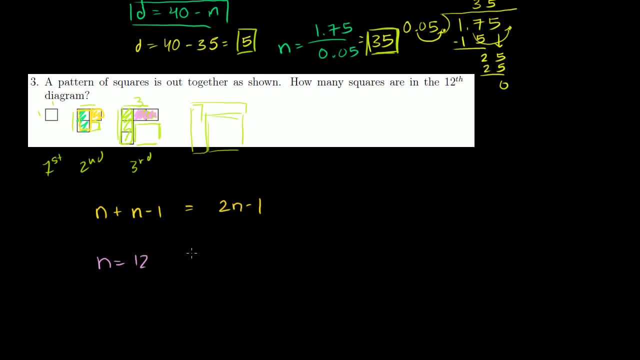 So the 12th square. so when n is equal to 12, it's going to be 2 times 12 minus 1,, which is equal to 24, minus 1,, which is equal to 23 squares in the 12th diagram. 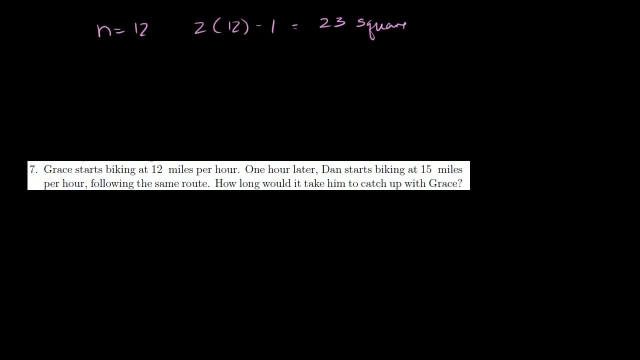 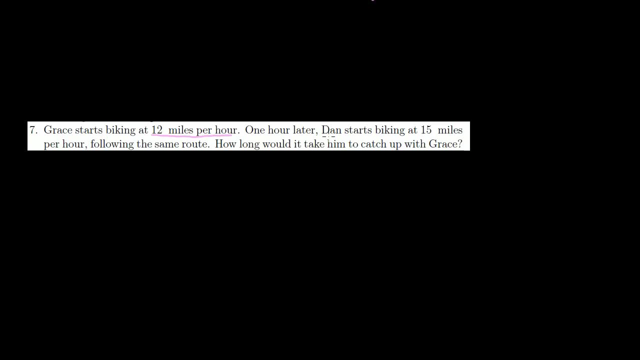 Actually I said let's do only one, Let's do another one. We're in the zone. Grace starts biking at 12 miles per hour. 1 hour 1 hour later, Dan starts biking at 15 miles per hour. 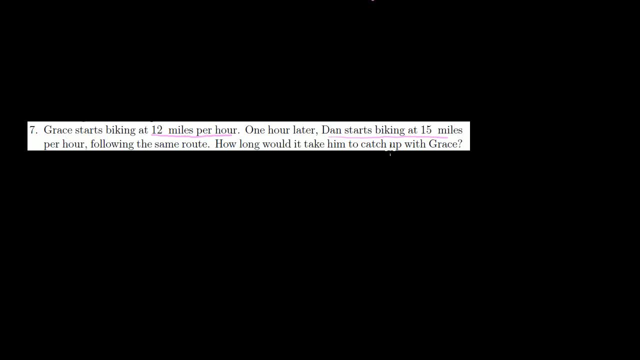 following the same route. How long will it take him to catch up with Grace? So let t equal time Grace The time Grace is biking. Actually, let me do it this way. Let me do it the time Dan is biking. Then how long will Grace be biking? 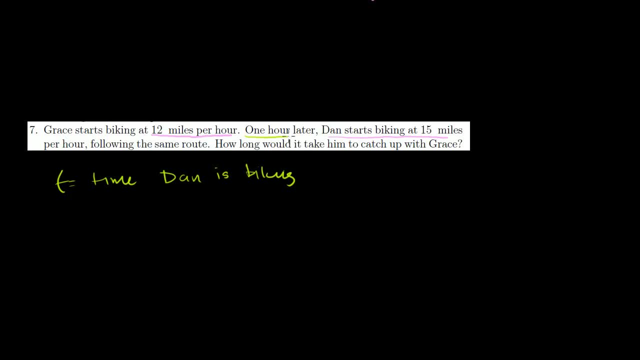 Well, When he starts an hour later, he starts. So whatever number this is, Grace is going to be biking for one more hour. So t plus 1 is equal to time Grace is biking. When this is 0, this is going to be 1.. 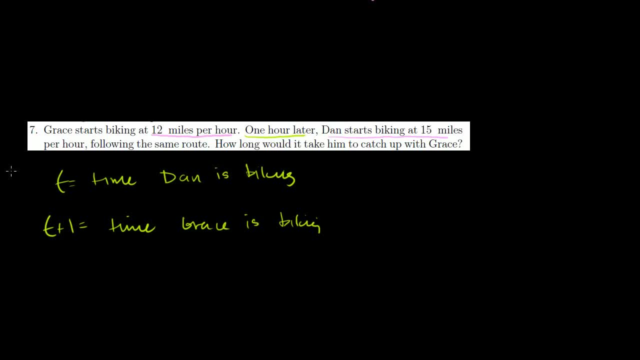 She would have already been biking for 1 hour, And we just have to remember that distance is equal to rate times time. So Dan's distance: 1.. Dan's distance is going to be equal to 15 miles an hour times the time in hours. 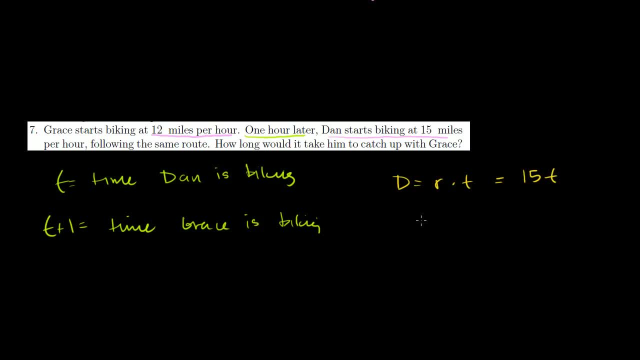 This is Dan's distance And then Grace's distance. Maybe I'll call that g, Or let's say d for Grace. That's her distance as well. That's, her distance Is going to be equal to 12 miles an hour. 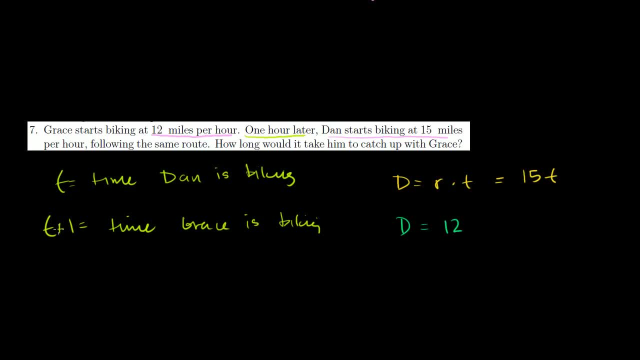 And her time in terms of t is going to be t plus 1.. She's going to always be traveling for one more hour than Dan, So 12 times t plus 1.. And the point at which they catch up, that's the point at which these two things 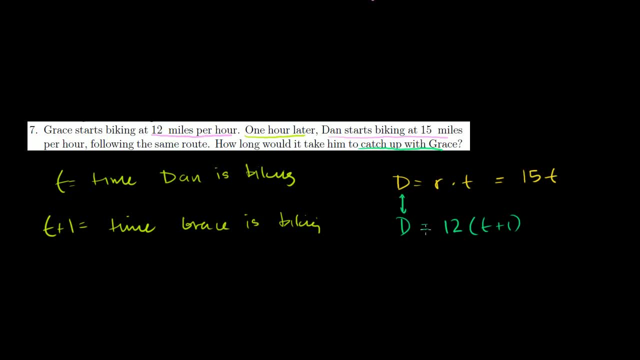 are going to be equal to That. Dan's distance is going to be equal to Grace's distance, So we just have to set these two to be equal to each other, So you get 15t is going to be equal to. That is how far Dan has been riding his bike. 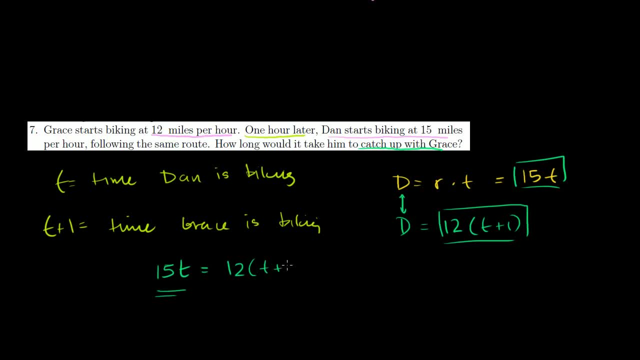 And then it's going to be equal to 12 times t plus 1.. That is how far Grace is. Grace has ridden her bike And remember her time is always going to be one hour more than Dan's, So let's just solve for time. 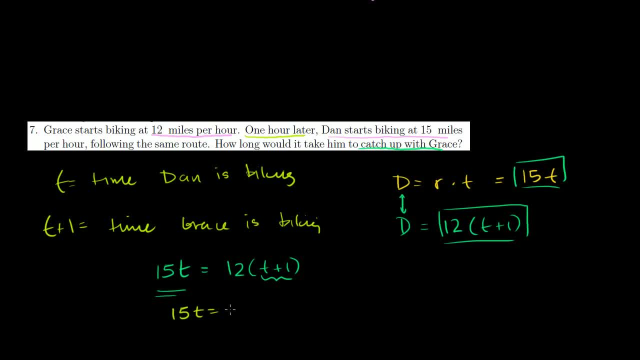 So we get 15t is equal to 12t plus 1.. And then if we subtract 12t plus 12.. Don't want to make a mistake there. If we subtract 12t from both sides, you get 3t is equal.